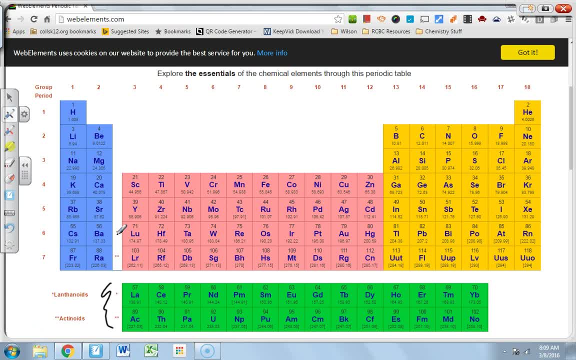 we have to first realize where they go in the periodic table. okay, Um, and different periodic tables show different things, but the periodic table is going to tell you exactly what that one, uh, believes. So you're going to put this: 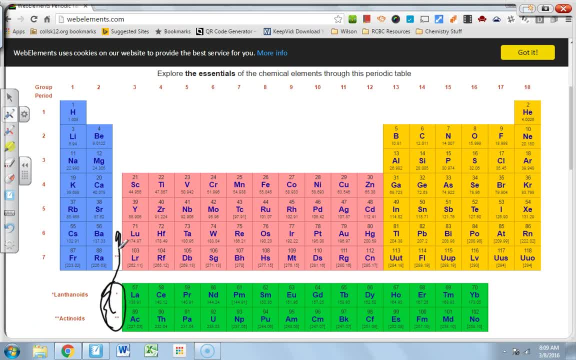 put these elements right here, okay. So imagine that periodic table stretched out and that in here are these 14 elements that go here. So when we do that, let's see we're going to do. um, let's say, element number 60, neodymium. Okay, so we're going to go down through. 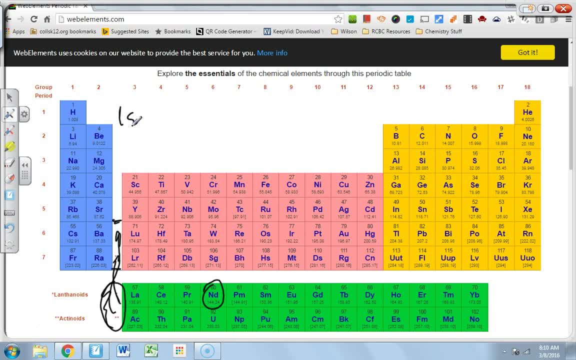 and we're going to start the electron configuration: 1s2, 2s2, 2p123456,, 2p6, 3s2,, 3p6, 3p6, and now let's see, the periodic table tells us to go to 4s. 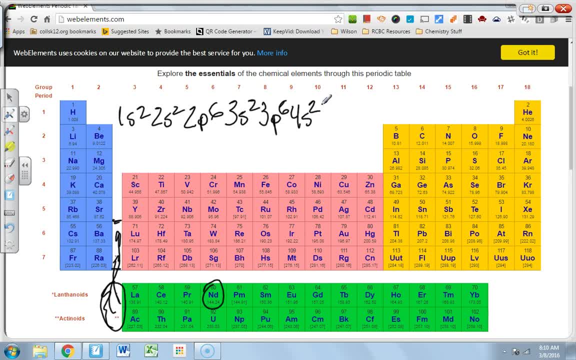 2s2, and then we go to 3,, 3d10, and then we go to 4p6, and now we go down to- I'm running out of room, so I'm going to go down here- 5s2, and then 4d10,, 5p6, and now we're at 6s2.. 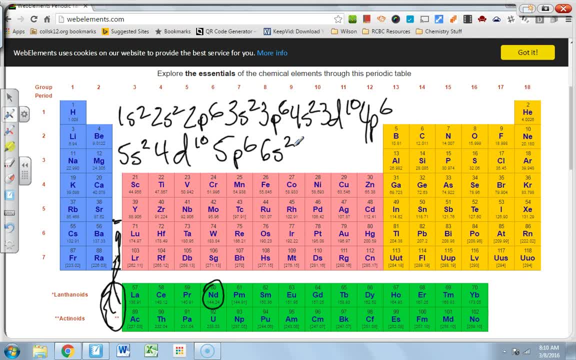 Now, where's the first time that you see F-electrons? We see them. let's see the first energy level, or? the first shell has just Ss. Okay, the second shell, the second energy level, has Ss and Ps, has two. The third energy level has three different: Ss, Ps and Ds. 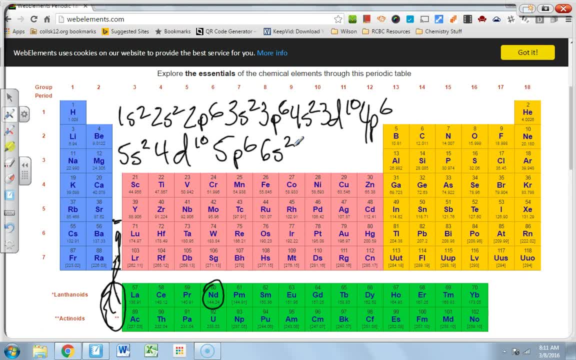 And so it's not until we get to the fourth energy level that we see the F-electrons. And so that's what this is. These are the four F-electrons, Okay, and then the actinides, or actinoids. 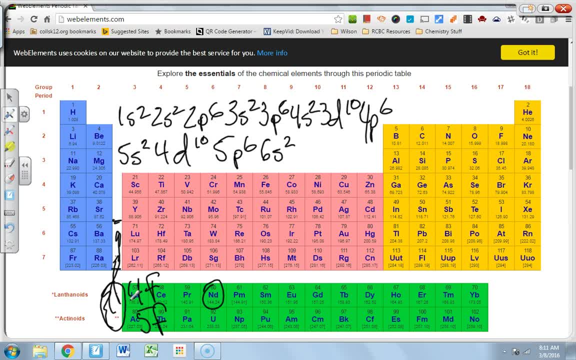 are the five F-electrons. So if we're going to neodymium, that's going to be 4F1, 2, 3, 4.. So we're going to do 4F4.. Okay, what if we go past that? What if we go to like something like? 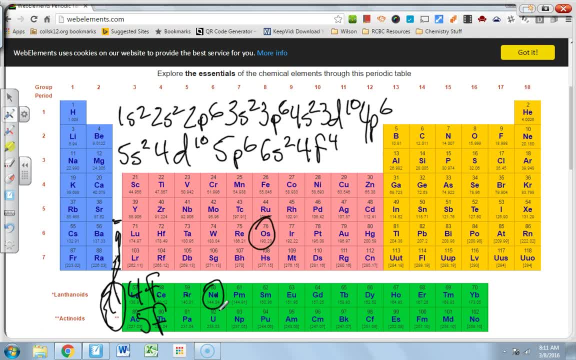 osmium. Okay, well, if we go to osmium we go through all the ones that we did with neodymium, except realize the four Fs now have 1,, 2,, 3,, 4,, 5,, 6,, 7,, 8,, 9,. 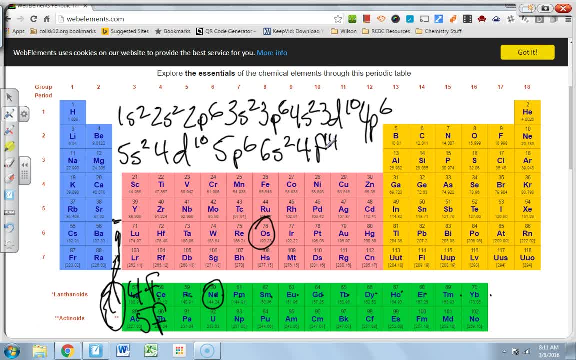 10,, 11,, 12,, 13,, 14.. And that makes sense because there's seven different F-orbitals, those double clovers. Each orbital can hold two electrons, so that's for a total of 14.. 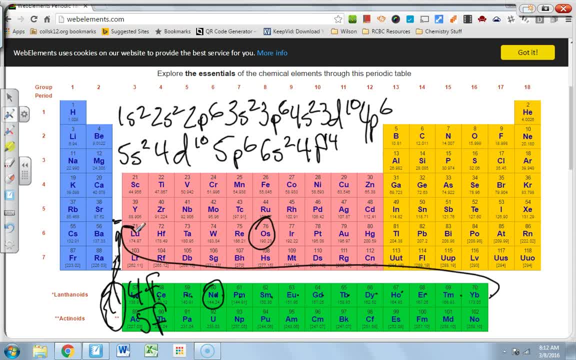 And now we come back up here, okay, using the atomic number on the periodic table. So we do, let's see here. So now we're here, and this is now the 5Ds. So that's 5D1.. 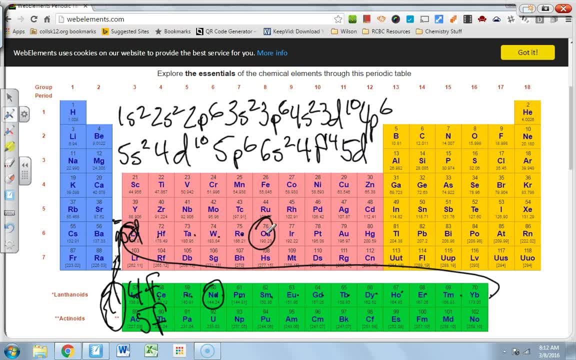 Okay, so now we're here, and this is now the 5Ds, So that's 5D1.. Okay, so now we're here, and this is now the 5Ds, So that's 5D1.. 1,, 2,, 3,, 4,, 5,, 6,, 5D6.. Okay, And so that helps us. 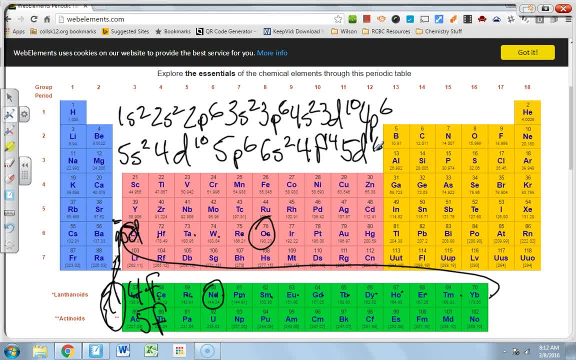 and so that helps us understand what the sections of the periodic table are. I go to web elements and use web elements because it color codes this. okay, And so that's how F-electrons are determined. should we try one more? okay, you could try it on your own, let me. 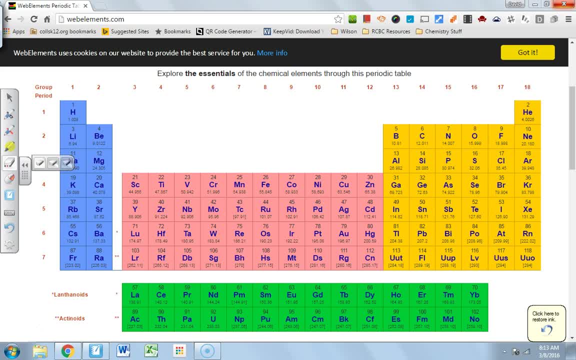 actually do it this way. I'll just, I'll just exit here and then I'll go back here, okay, so now let's pick another one, let's pick. let's pick that one. okay, that is protactinium. let's let's do a shortcut, okay, instead of going down through all the all the. 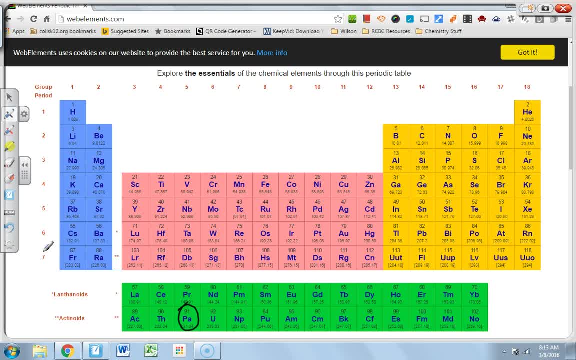 filled electrons. let's just start here, so we know that it's going to be one s two, two s two, two p six, three s 23 p. six. four s two, three d ten, 4 p, 65 s, 2, 4d, 10, 5 p 6. 7 p 6, 1 n, 5 p 6, 7 p 6, seven ap 3Z 6 p 6a 3b morning 7, 2, 7 p 2, 3 p 5xter. but Ally, yeah, we appear a winsan nettle.